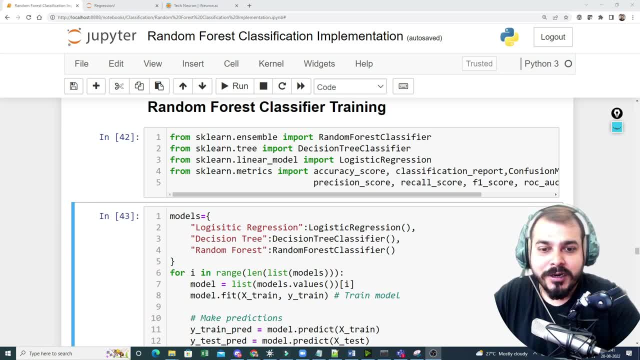 probably perform the hyperparameter tuning. Okay now, it is always a good practice. if someone says that, Krish, like, if you are solving a machine learning problem, statement which algorithm do you select? My always the answer will be that try each and every machine learning algorithm and then try to find out the performance metrics and, based on this performance metrics, take a. 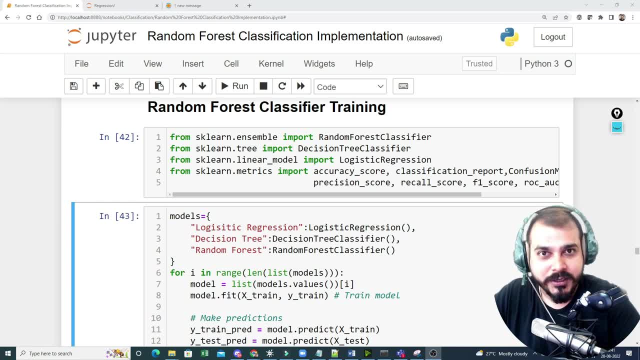 decision of which algorithm you're going to select and perform hyperparameter tuning. Okay, so here I will just give you an example. Okay, this is one of the project that I'm actually creating. It is a complete end-to-end project. If you probably want this entire end-to-end project, at least give 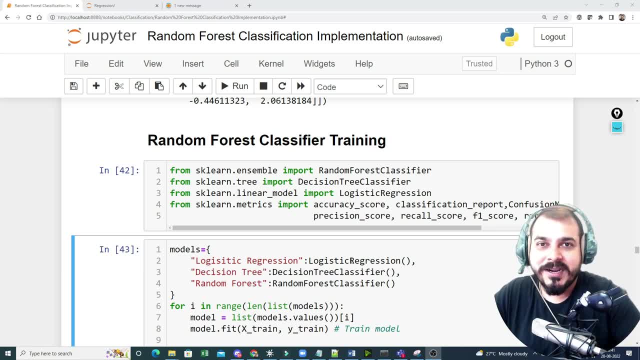 thousand likes on this video and this particular project. I'll try to upload it Because this project completely it is going to build on CI CD pipelines and all. So I'm working on that. So make it thousand likes, I will definitely upload this entire project. step. 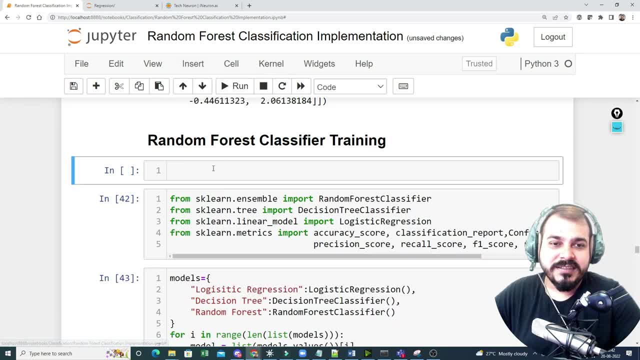 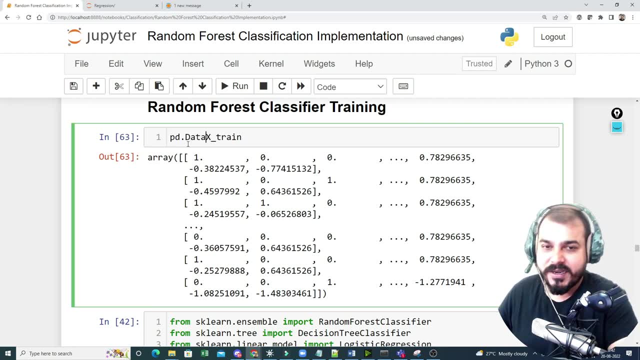 by step. Okay, and probably also going to have some live sessions. Now, let's say, this is my Xtrain data. Okay, so these are some of the features that I have in Xtrain data. So, let's say, if I write PD dot data frame, you will be able to see how many number of features are there. And 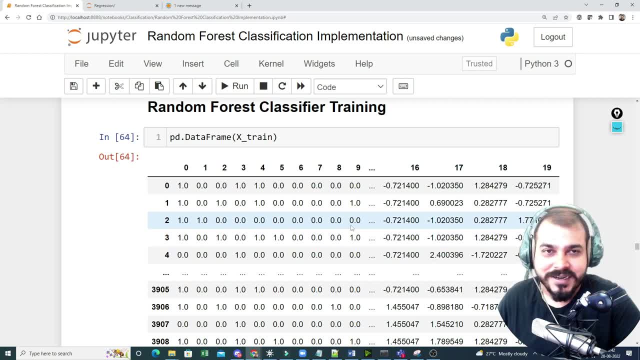 I did an extensive feature engineering and lot, many things I did Okay on to this. So I did feature engineering, I probably did categorical encoding, binary encodings, many such things Okay, and finally I was able to get all these things. But my main aim is to show you an 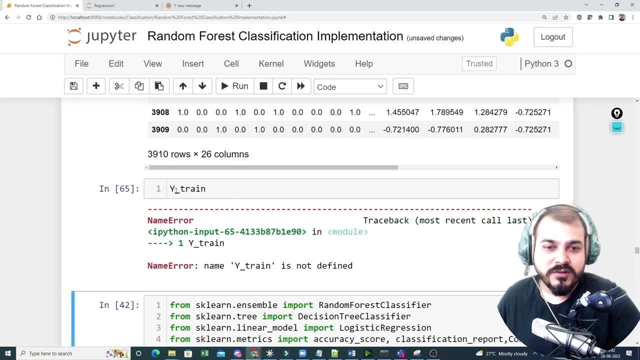 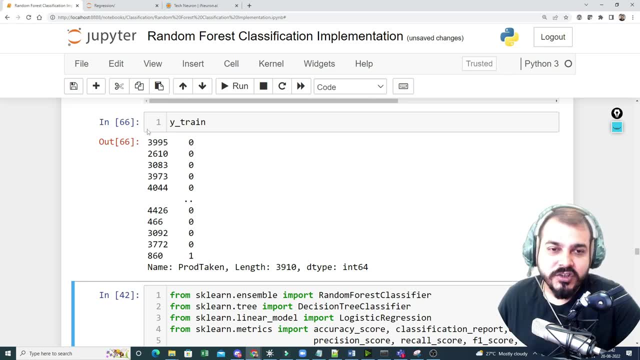 efficient way of training a model. So this is my Ytrain. Okay, so Ytrain is nothing, but it is a binary classification And it is one more problem statement which I'm solving. It is a multiclass classification. So here what I'm actually going to do now. I definitely want to try many models. 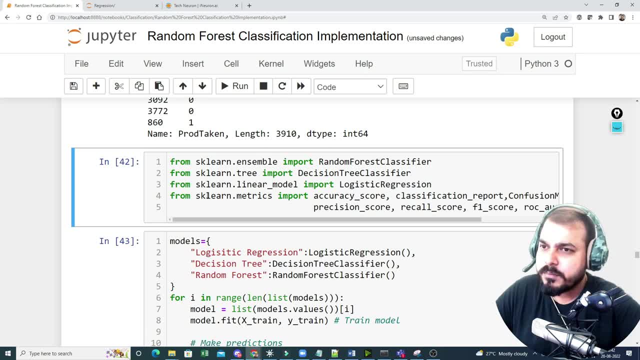 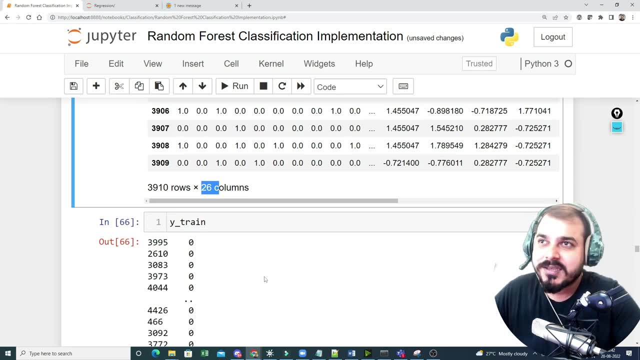 And obviously for you right, whenever you have a big data with many number of dimensions- Because here also you have somewhere around 26 dimensions, 26 columns, right? You cannot just say that, okay, this algorithm is going to perform. So let's take one example. So first of all, I have 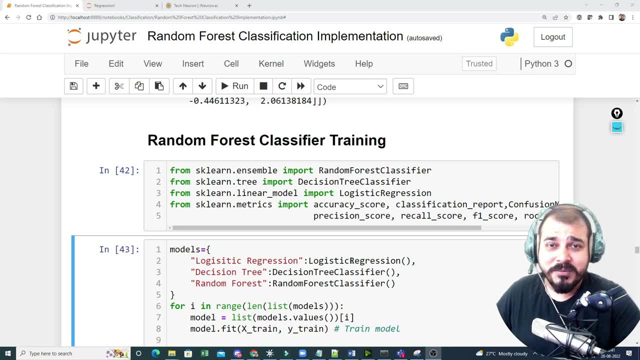 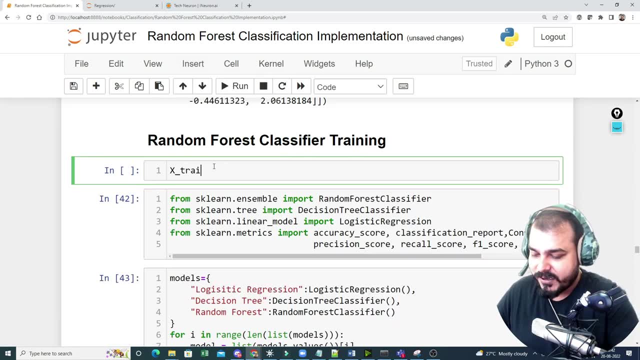 So I am working on that. So make it 1000 likes. I will definitely upload this entire project step by step, And probably we are also going to have some live sessions. Now, let's say, this is my X-Train data. So these are some of the features that I have in X-Train data. 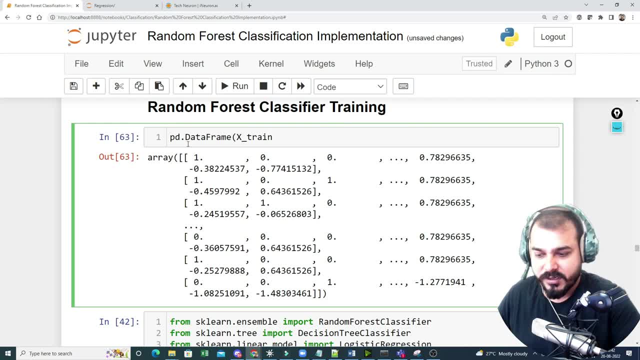 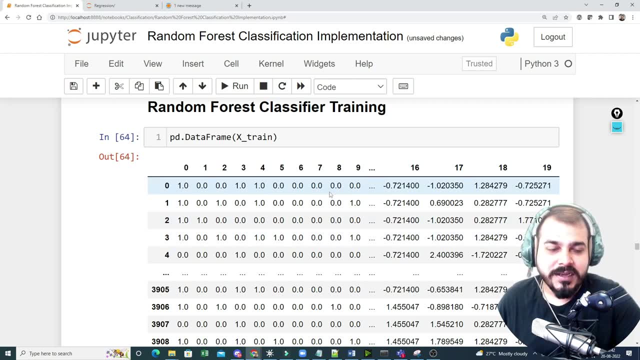 So, let's say, if I write pddataframe, you will be able to see how many number of features are there. And I did an extensive feature engineering and lot, many things I did Okay on to this. So I did feature engineering, I probably did categorical encoding, binary encodings, many such things. 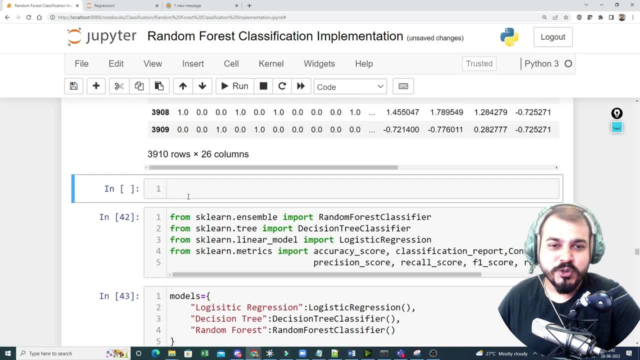 Okay and finally, I was able to get all these things, But my main aim is to show you an efficient way of training a model. So this is my Y-Train. Okay, so Y-Train is nothing, but it is a binary classification. 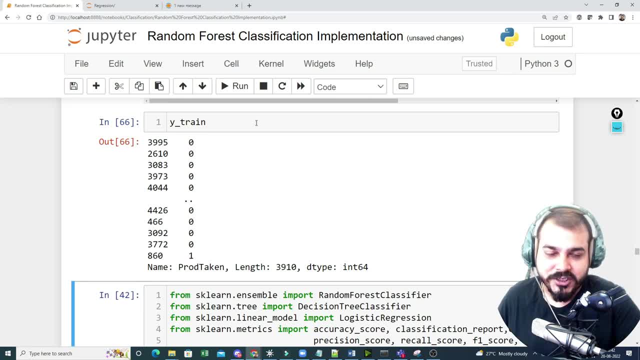 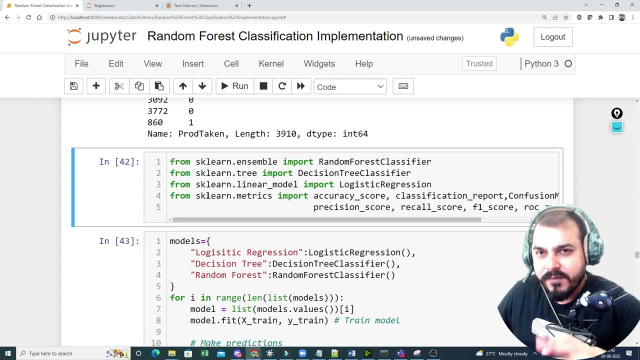 And it is one more problem statement which I am solving. It is a multi-class classification. So here what I am actually going to do now. I definitely want to try many models And obviously for you right, whenever you have a big data with many number of dimensions. 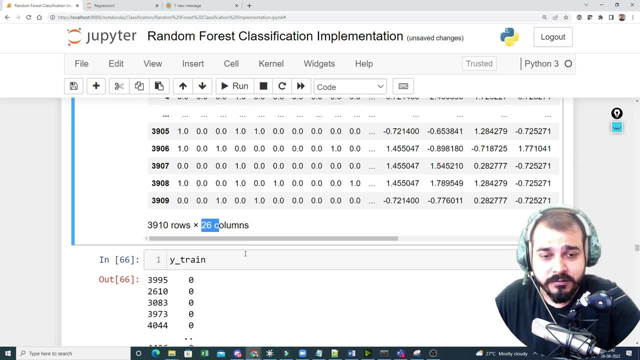 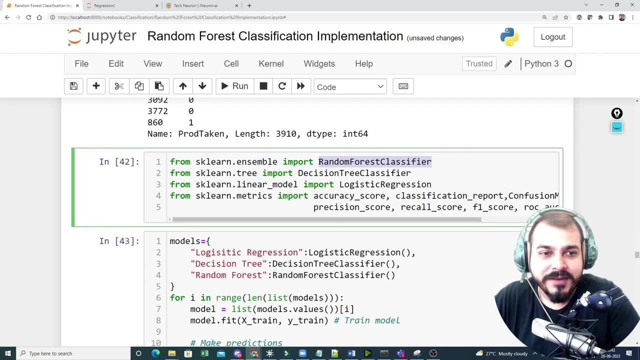 Because here also you have somewhere around 26 dimensions, 26 columns, right? You cannot just say that, okay, this algorithm is going to perform, So let's take one example. So first of all, I have imported a random forest classifier decision tree logistic regression. 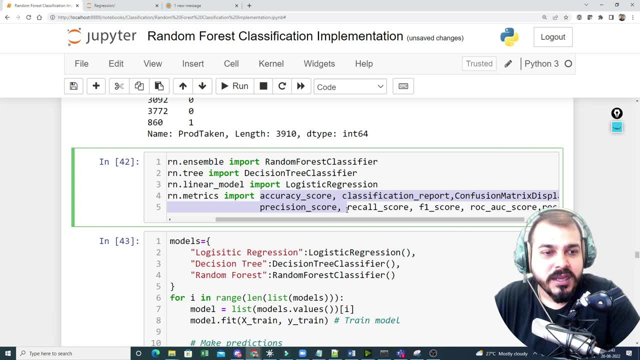 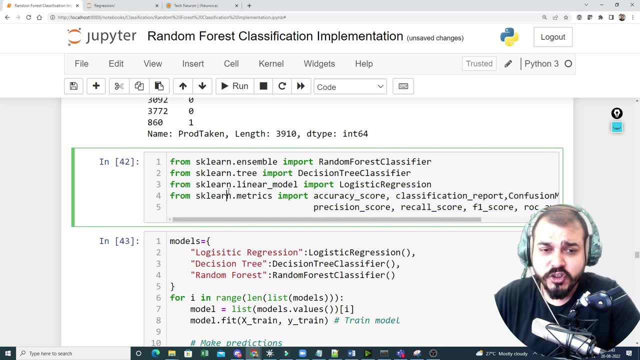 Along with that, you can see I have accuracy score classification report, precision recall score, recall score, F1 score, RUAC score. Every scores are over here. Now what I am actually going to do, I will just import this. 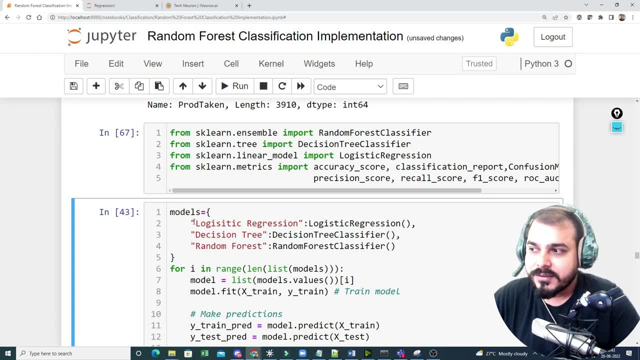 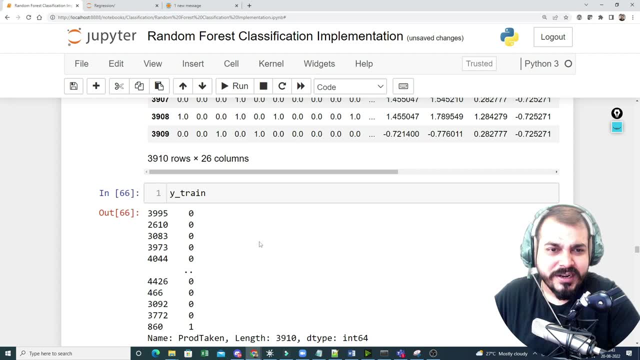 And now the thing that I am going to apply. see, Over here you can definitely create a pipeline right And pipeline. also, you will try to add, like how to do the transformation, and all That part is already done. I have already taken care of that. 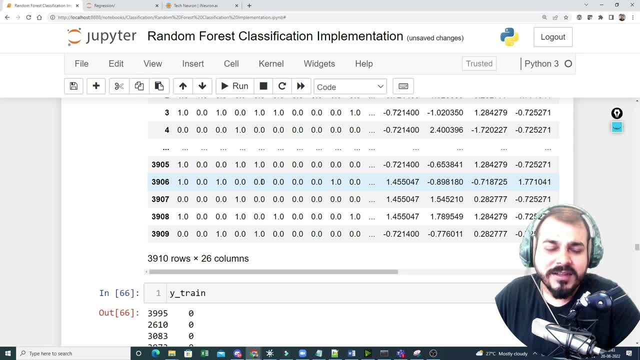 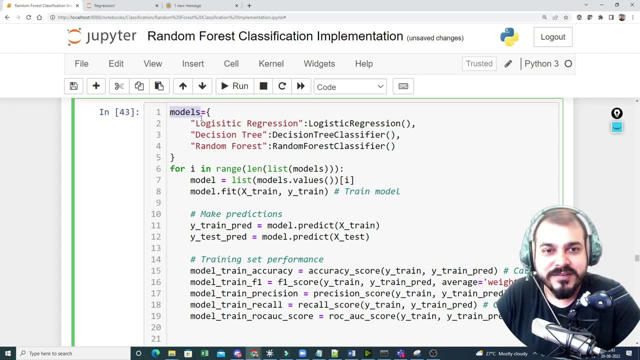 And probably in some of the videos I can also show you how to do column transformation and all. But here, how many machine learning algorithms I am going to train, I am going to show you. See, here I have created a dictionary, which is with the name models. 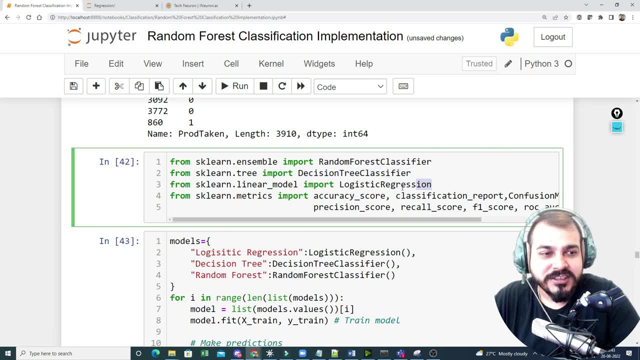 imported random forest classifier decision tree, logistic regression. Along with that you can see I have accuracy score classification report, precision recall score, recall score, F1 score, RUC score. Every scores are over here. Now what I'm actually going to do, I'll just import this. 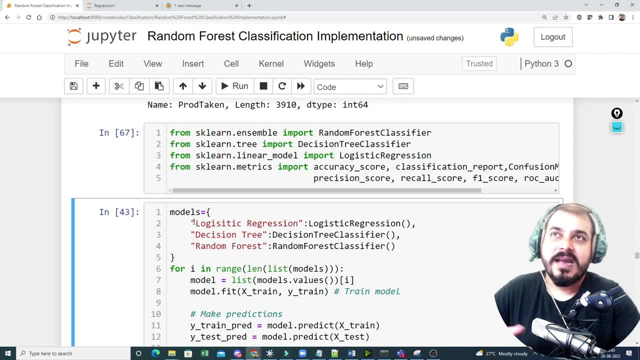 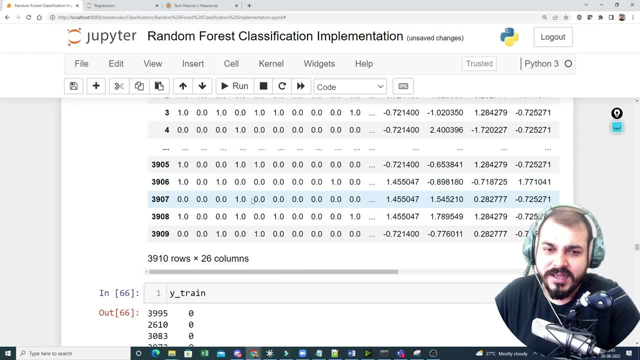 Over here you can definitely create a pipeline, right And pipeline. also. you'll try to add, like how to do the transformation and all That part is already done. I have already taken care of that And probably in some of the videos I can also show you how to do column transformation and all But. 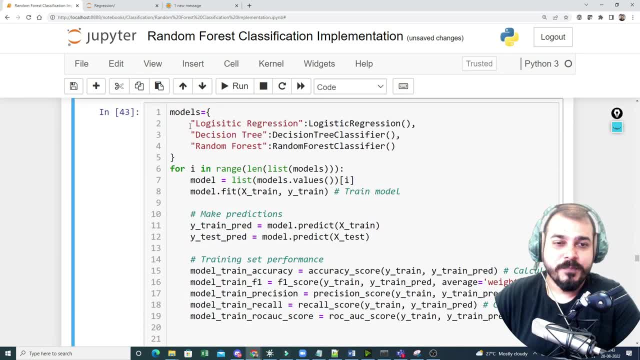 here how many machine learning algorithms I'm going to train. I'm going to show you See, here I've created a dictionary which is with the name models And here you can see I have key value pairs like logistic regression- Here I have logistic regression. Decision tree. Here I have decision tree classifier. 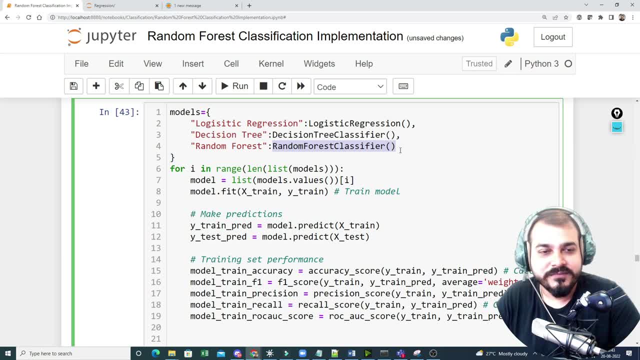 The random forest And here I have a random forest classifier. OK, so here you can basically say that key value pairs with respect to different, different algorithms. I have just taken. OK, now see how well this looks. OK now, when I did, for i in range of length of list of models. So you know that. 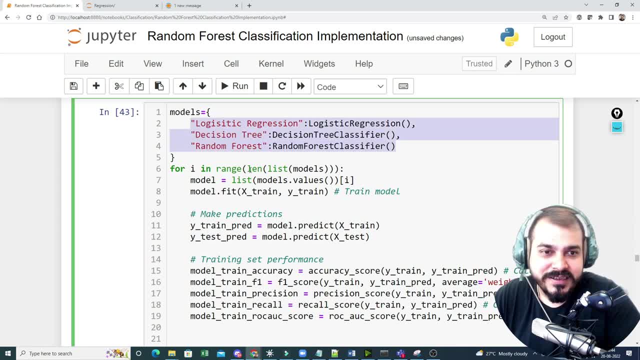 how many models you are going to get over here: Three right. When you do list of models and find out the length, you are going to get three Right. so we'll take the first model based on the iteration i value, And then we'll do the fit on equal. 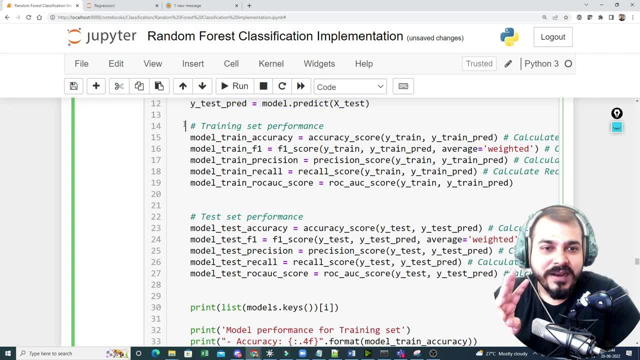 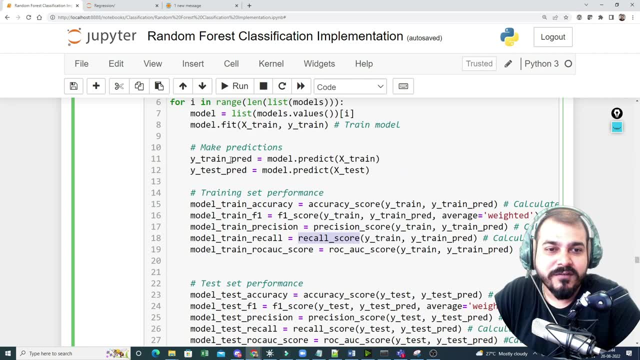 train and y train and then we'll do the prediction. then we'll get the training set: performance, accuracy, like accuracy score, f1 score, precision, recall score, everything based on the predicted values that you have got from the training data. similarly, you'll get the test set performance. so 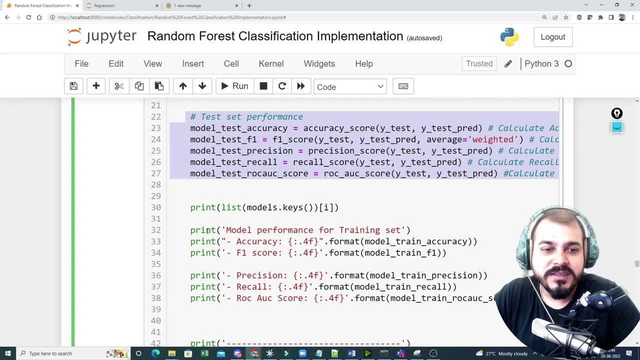 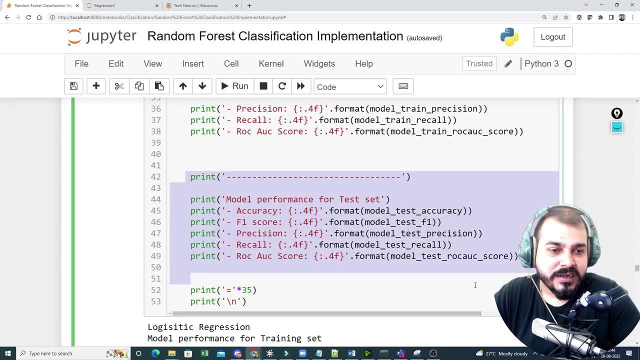 here also, you'll try to get the with respect to the test- how was the performance? and, finally, you'll print all the details over here with respect to training and test data set and, similarly, the test data. you are printing it over here. okay, so let's say, if i execute this, that basically means 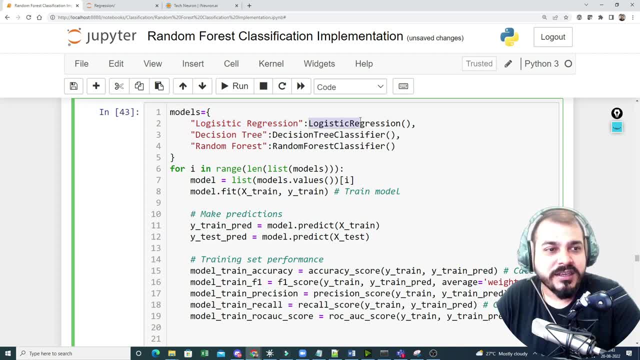 And here you can see I have key value pairs like logistic regression- Here I have logistic regression. decision tree- Here I have decision tree classifier. Random forest And here I have random forest classifier. Okay, So here you can basically say that key value pairs with respect to different, different algorithms I have just taken 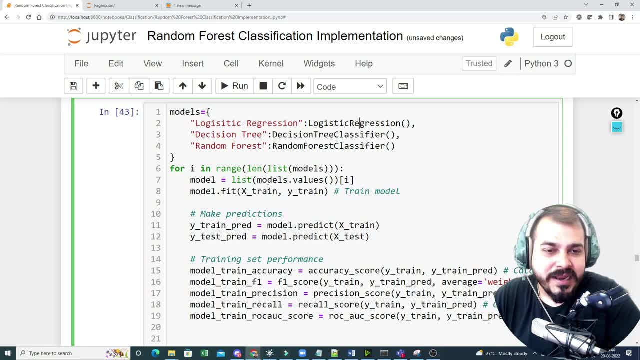 Okay, Now see how well this looks. Okay Now, when I did, for I in range of length of list of models. So you know that how many models you are going to get over here, Three right. When you do list of models and find out the length, you are going to get three right. 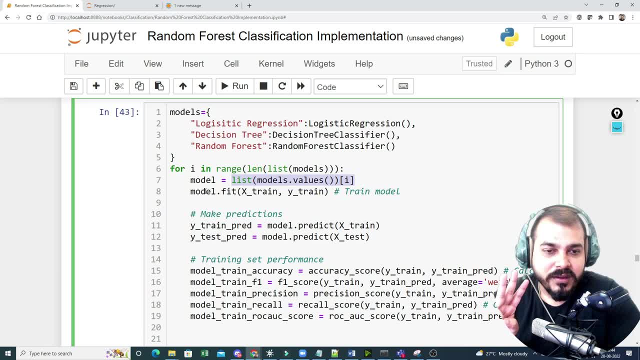 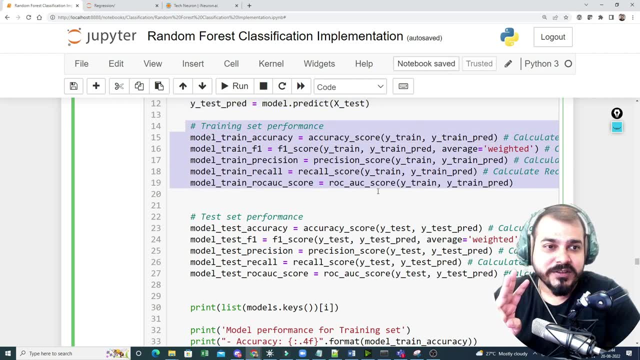 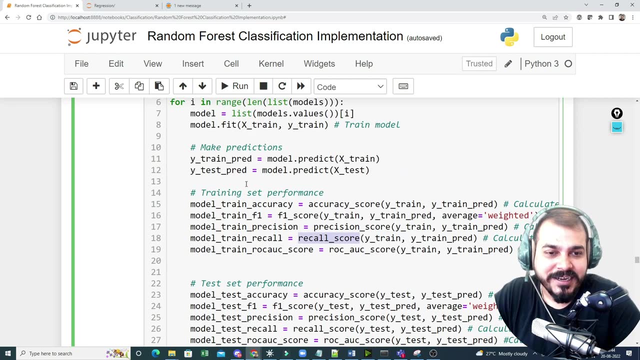 So we will take the first model based on the iteration I value, And then we will do the fit on And then we will do the prediction, Then we will get the training set: performance, accuracy, like accuracy score, F1 score, precision, recall score, everything based on the predicted values that you have got from the training data. 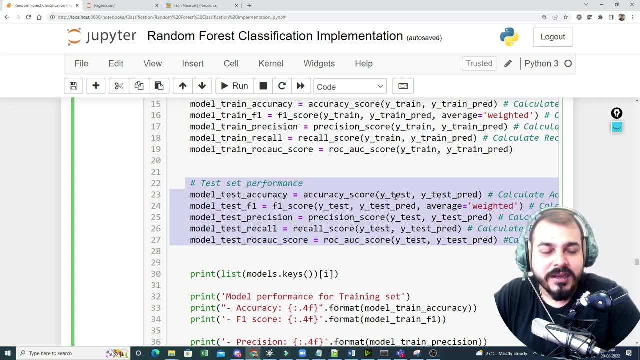 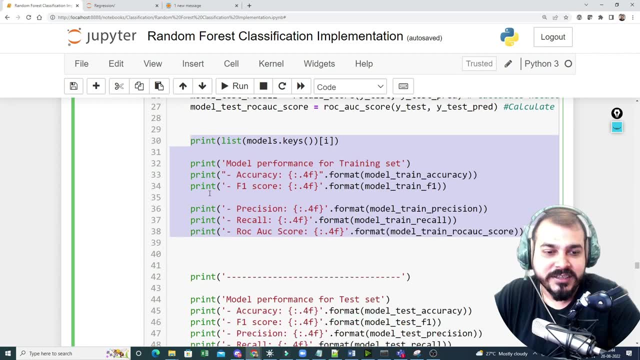 Similarly, you will get the test set performance. So here also you will try to get the with respect to the test: how was the performance? And finally, you will print all the details over here with respect to training and test data set. 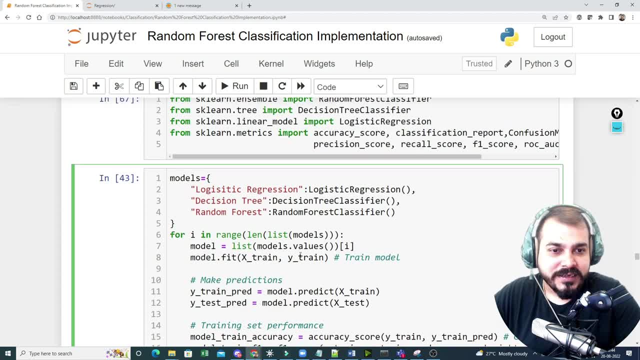 And similarly the test data. you are printing it over here, Okay. So let's say, if I execute this, That is the test set, Okay. So that basically means I am going to get three model information. One is logistic decision tree: random forest. 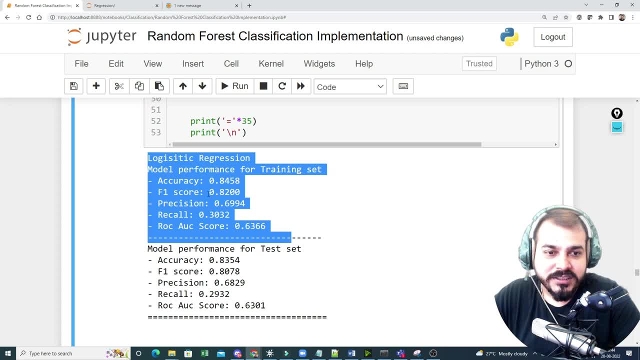 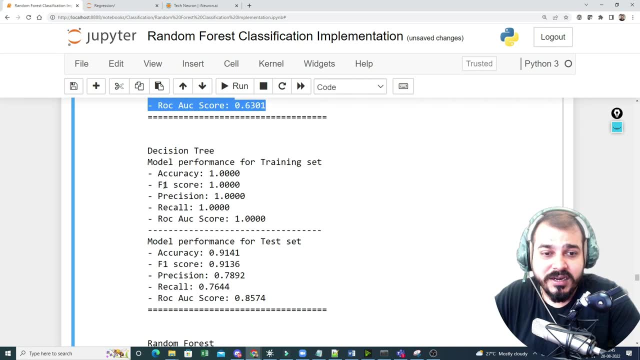 So once I execute it, here is how your model looks like. See with logistic: obviously you are going to get less accuracy With for the test data also, you see less accuracy, But decision tree and all it is trying to overfit over here. 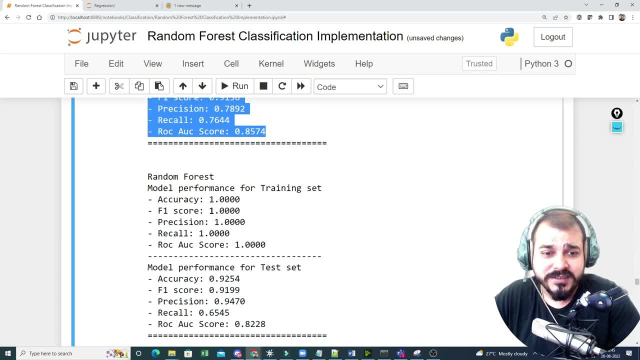 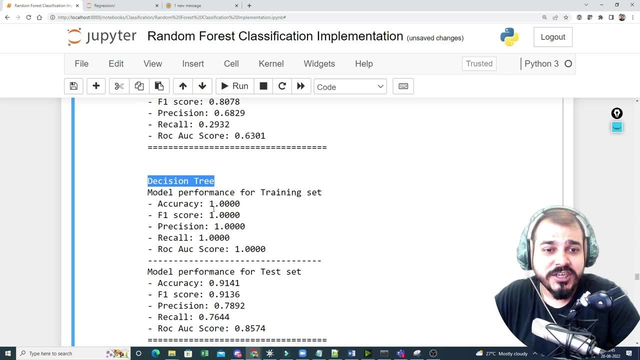 And here, with respect to the test data, yes, the accuracy is good. Recall is 0.76.. And here, random forest also. you are getting a good accuracy. Now, out of this, now you have an option. should we go with decision tree or should we go with random forest? 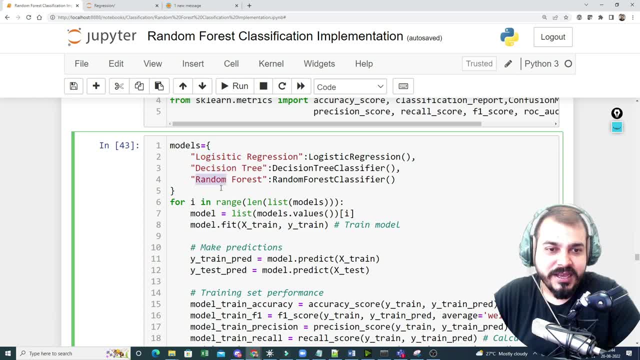 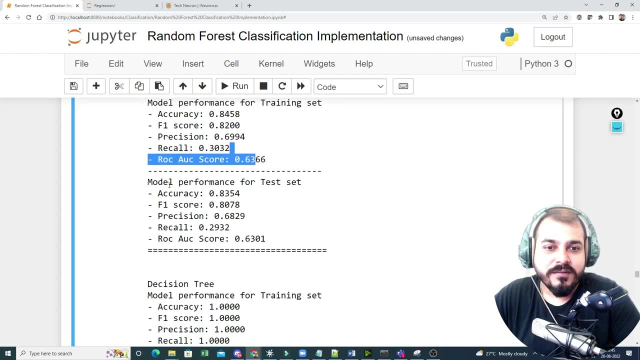 i'm going to get three model information. one is logistic, decision tree, random forest. so once i execute it, here is how your model looks like. see with logistic. obviously you're going to get less accuracy with uh for the test data also, you see less accuracy, but decision tree and all it is. 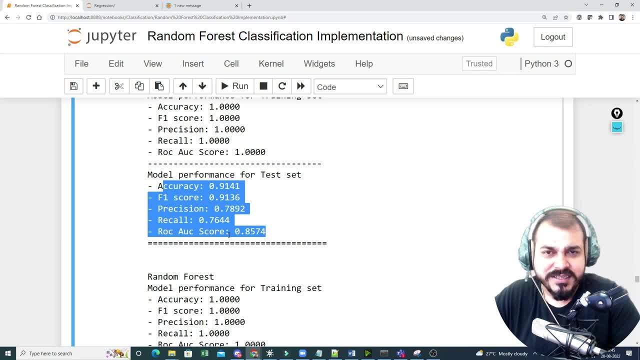 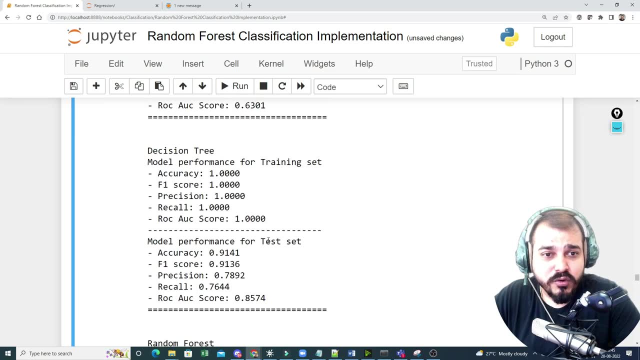 trying to overfit over here and here. with respect to the test data, yes, the accuracy is good. recall is 0.76 and here, random forest also. you are getting a good accuracy. now this: now you have an option: should we go with decision tree or should we go with random forest? 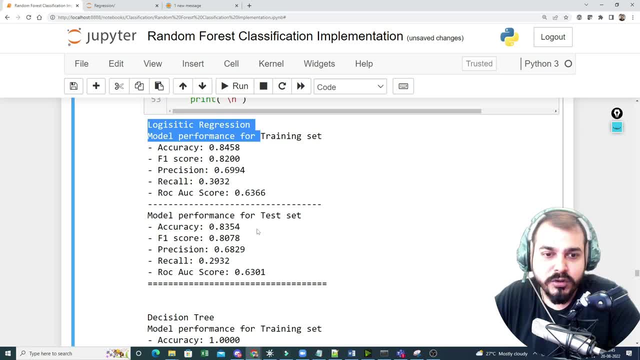 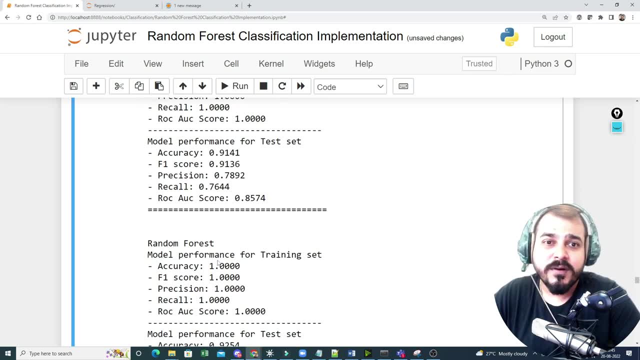 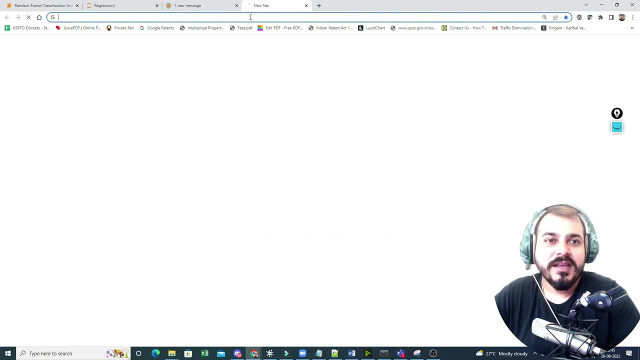 obviously you can ignore logistic regression because logistic regression, even though you perform many hyper parameter tuning, it is not going to work. but with respect to decision tree and random forest, you can basically use this and perform hyper parameter tuning. so in the next step, what you do? you take up a random forest hyper parameter and this obviously from where you'll get. 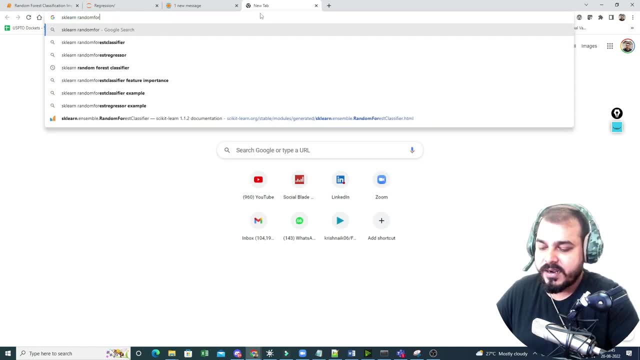 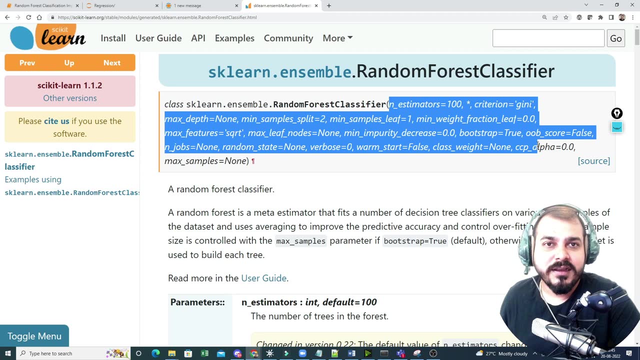 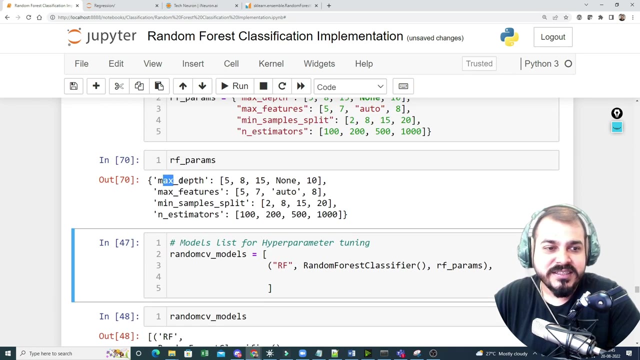 you'll get it from sk learn. so if i write sk learn- random forest classifier, you'll get all the parameters over here, right? where are the parameters? this is all parameters you can play with, right? so here i have selected some hyper parameters, so i have executed this. we executed this. now i'm going to try with this kind. 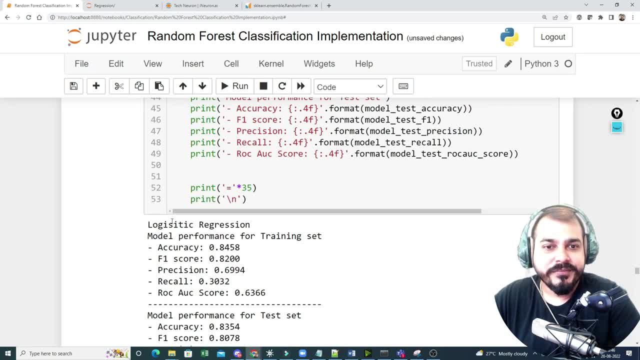 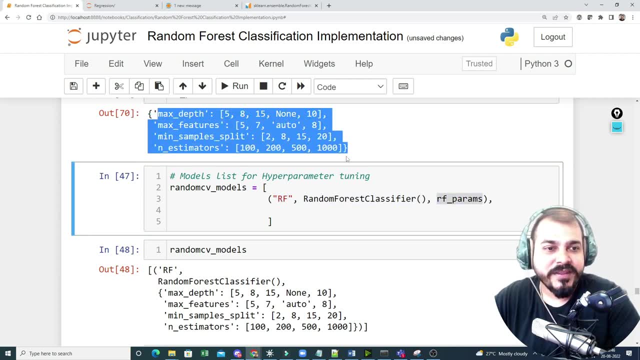 of hyper parameters in the similar way, like how we did it over here, right? so what i'm going to do? i'm going to select this. okay, i? i've used all the random forest parameters over here. similarly, i can make this similar parameters with decision tree and also create it over here in the same way. 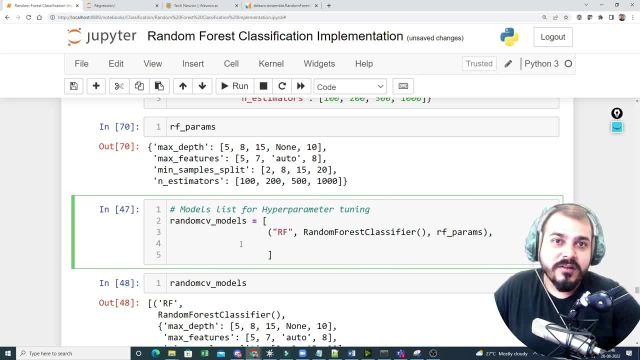 so what is exactly happening is now: you can try any number of parameters, you can try any number of models that you want, and this is the exact way you should basically perform with respect to training the model. don't do it. independent training for everyone at once. take up all. 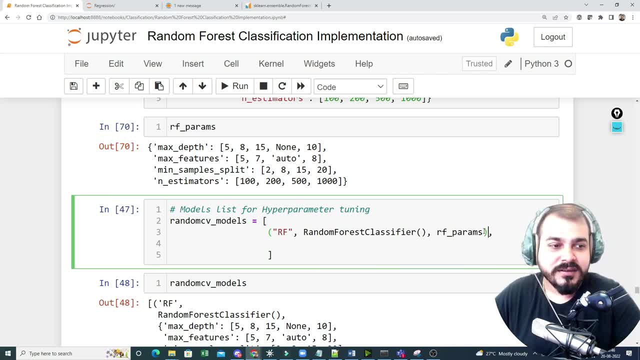 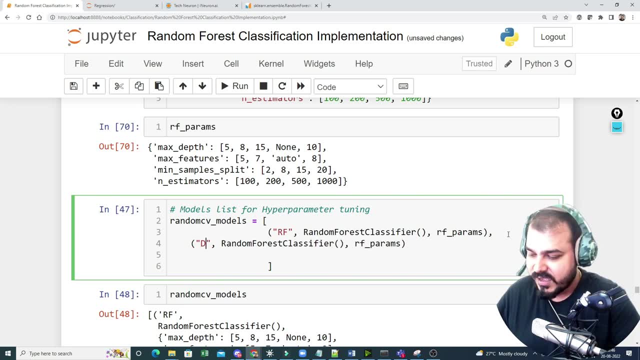 the training right. so here now i've taken the random forest. now probably you want decision tree, just go over here, paste it over here. use decision tree. use decision tree classifier like decision tree over here with my name and decision tree classifier and probably use the decision tree. 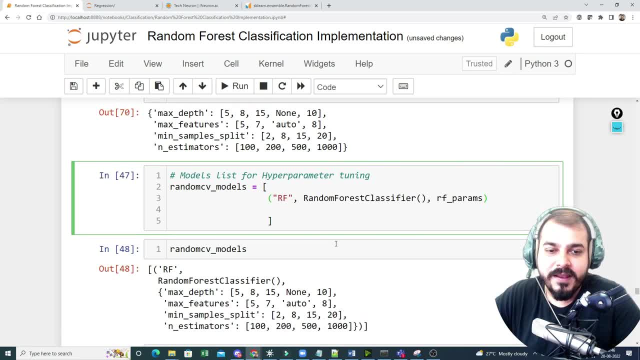 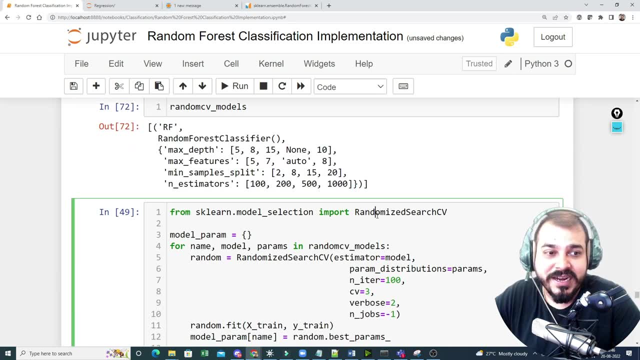 parameters. this is just to show one example. i've used random forest. okay, if you probably execute this and if you see this, here is what i'm going to try now see in the training stage what will happen here. i'm using randomizer cv. okay, so for name under so comma. 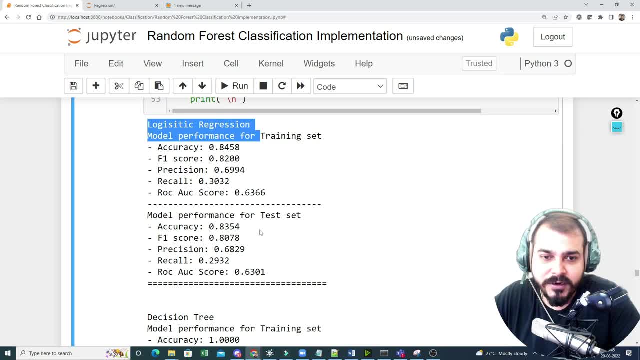 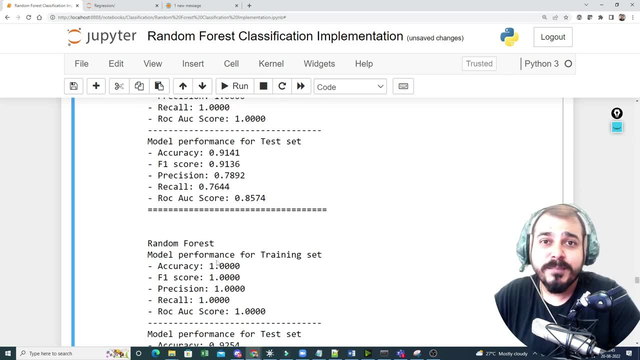 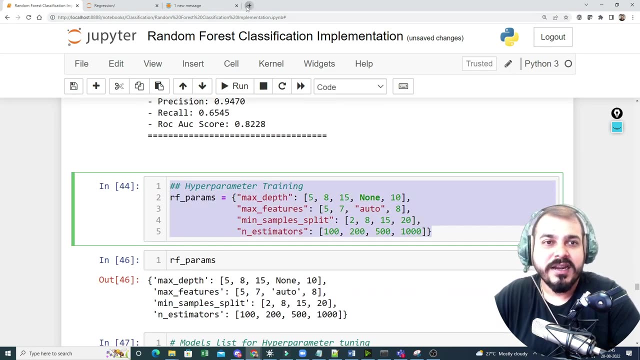 Obviously you can ignore logistic regression because logistic regression, even though you perform many hyperparameter tuning, it is not going to work. But with respect to decision tree and random forest, you can basically use this and perform hyperparameter tuning. So in the next step, what you do, you take up a random forest hyperparameter and this obviously from where you'll get? you'll get it from sklearn. 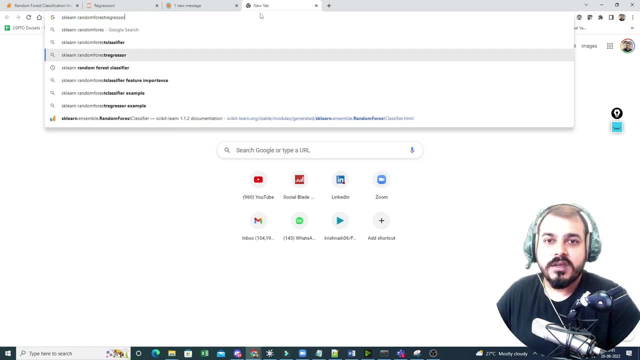 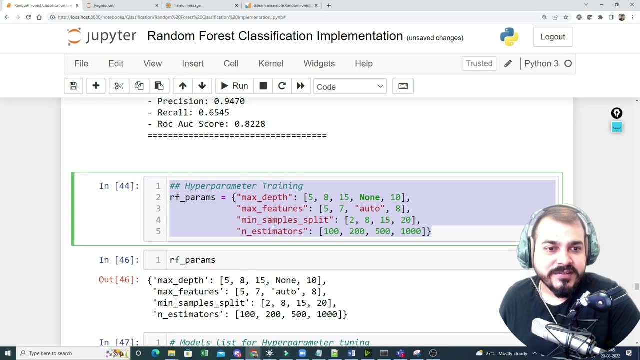 So if I write sklearn- random forest classifier, you'll get all the parameters over here, right? Where are the parameters? These are all parameters you can play with, right? So here I have to do this. I have selected some hyperparameters. 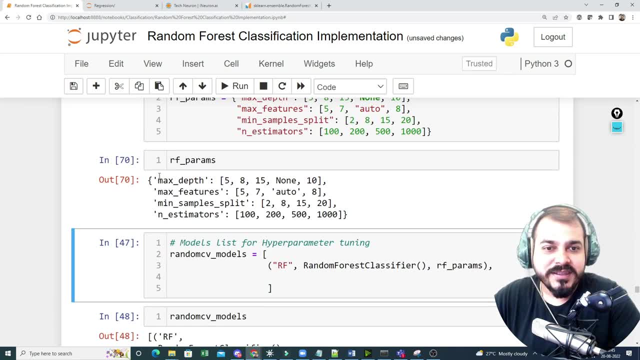 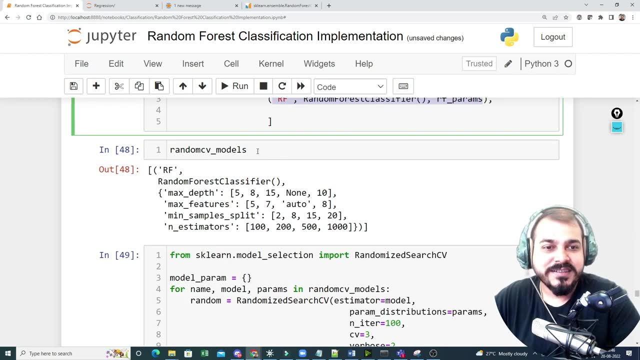 So I have executed this, executed this. Now I'm going to try with this kind of hyperparameters in the similar way, like how we did it over here, right? So what I'm going to do, I'm going to select this, okay. 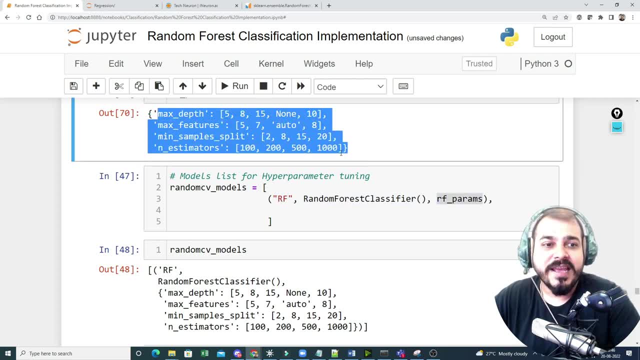 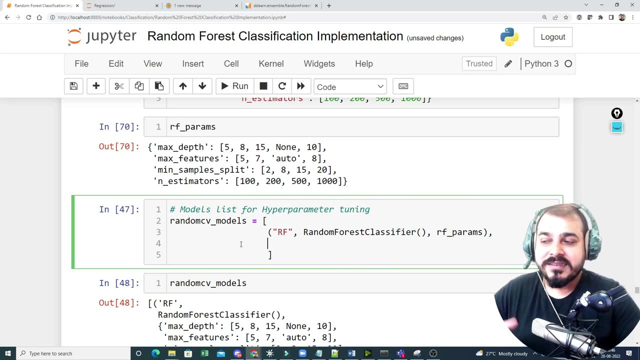 I've used all the random forest parameters over here. Similarly, I can make this similar parameters with decision tree and also create it over here in the same way. So what is exactly happening is now you can try any number of models that you want. 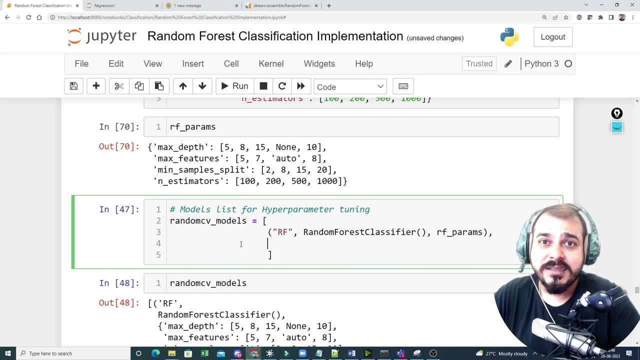 And this is the exact way you should basically perform With respect to training the model. don't do it. independent training for everyone at once. take up all the training right. So here now. I've taken the random forest. now probably you want decision tree? just go over here. 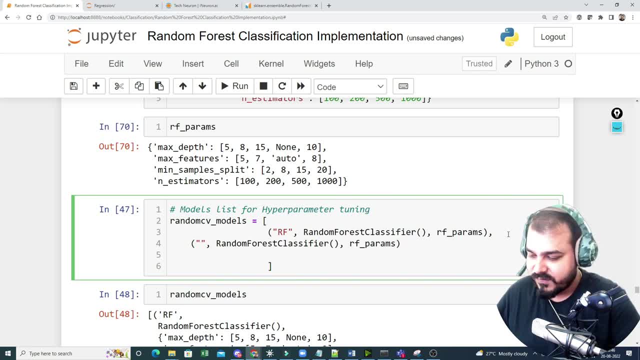 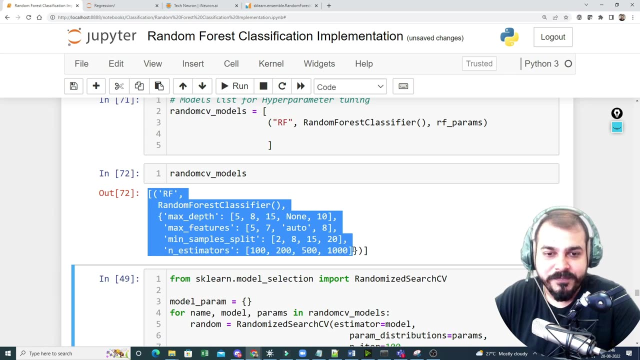 paste it over here. use decision tree. use decision tree classifier like decision tree over here with my name and decision tree classifier and probably use the decision tree parameters. This is just to show one example. I've used random forest. okay, Now, if you probably execute this and if you see this, here is what I'm going to try. 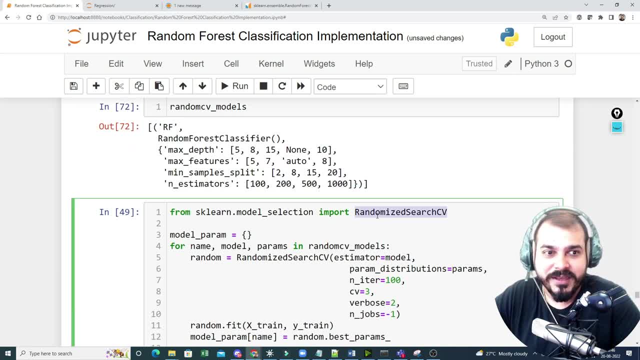 Now see in the training stage what will happen Here. I'm using randomized search CV, okay, So for name model params. so from this I'm getting the name, I'm getting the model, okay, When I'm iterating through this list and I'm getting the parameters. 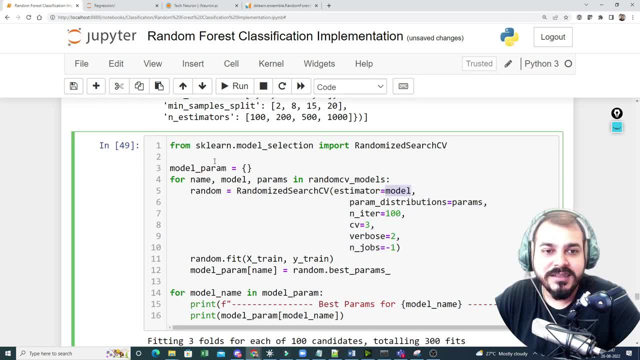 Now I can train my model with the randomized search CV. Here I'll just assign the model: which value is coming from here, params is coming from here, iteration and all we can play with it. And then we do the fit on X train, Y train and finally we got the parameters right. 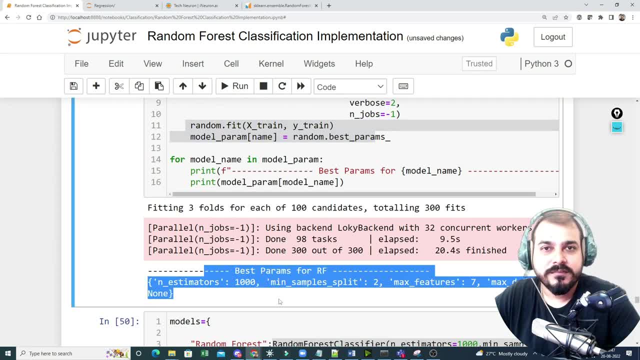 And once you execute this, you can see that, okay, Once you execute this, we'll get the best params score right, And then I can probably use this and train my model And, at the end of the day, see here also what I've done. 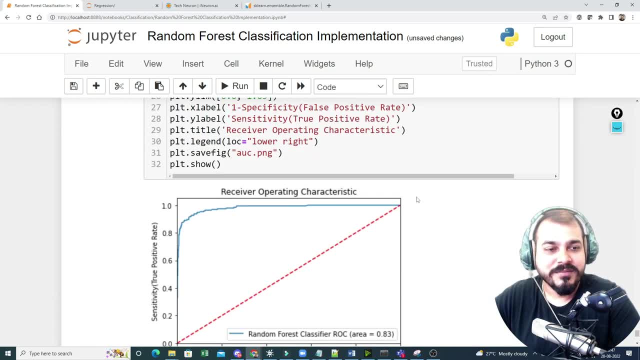 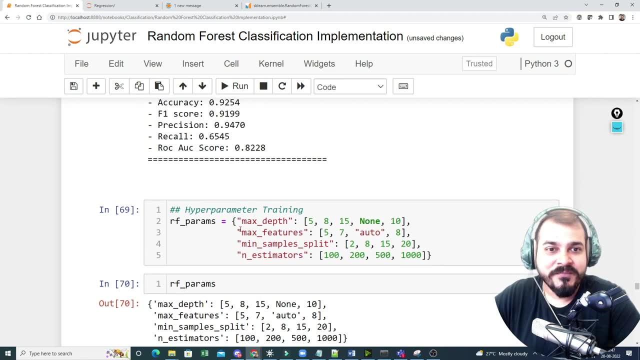 I've made this ROC ROC score also automated, So here you can see how amazing it is basically coming okay. So, and these are all projects right- This was basically developed from one of the FHDS batch, student right Who are right now working in iNeuron. 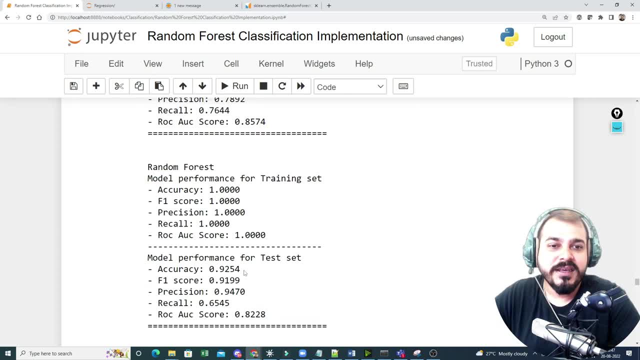 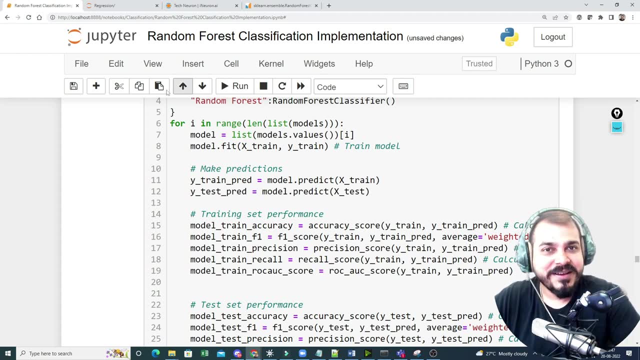 And since we are creating materials over here, you can see how beautifully they have actually explained it right Over here. And if you really want this entire end-to-end project, just make sure that you hit like make it thousand, But this is how you have to do. 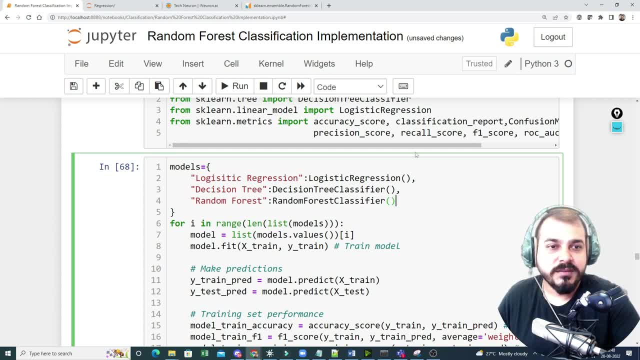 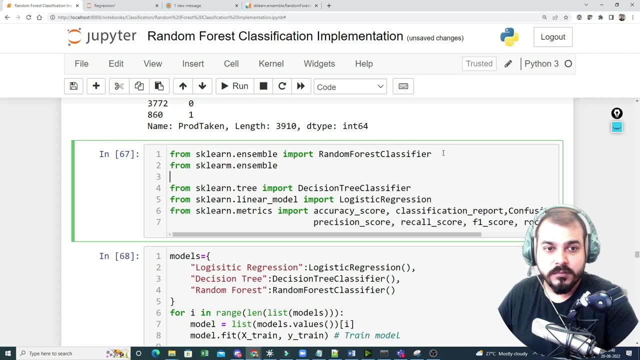 Tomorrow, if you want XGBoost, I will probably go and search for XGBoost. Suppose I want gradient boost, So I'll write from sklearnnsymbol- nsymbol- import gradient boost. classifier right, So I can actually go for gradient boost. 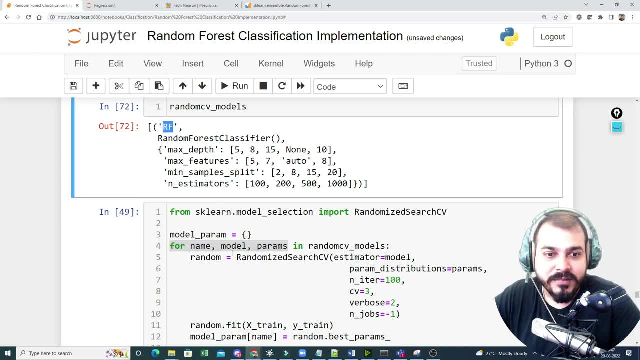 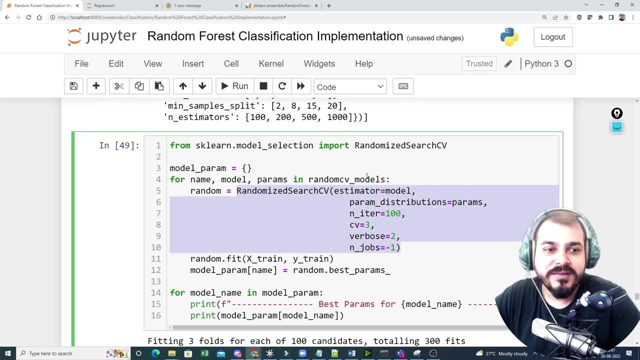 model: comma, param. so from this i'm getting the name, i'm getting the model, okay, when i'm iterating through this list and i'm getting the parameters. now i can train my model with the randomizer cv. here i'll just assign the model: which value is coming from here? params is coming from here. 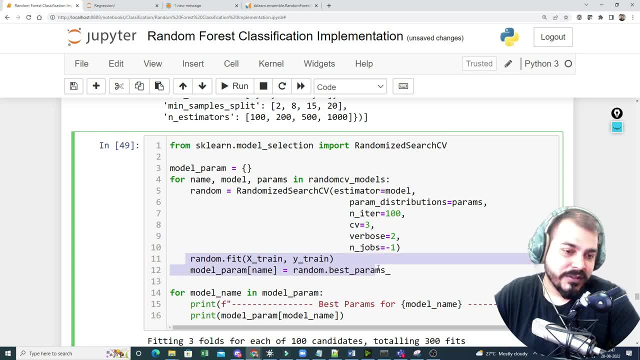 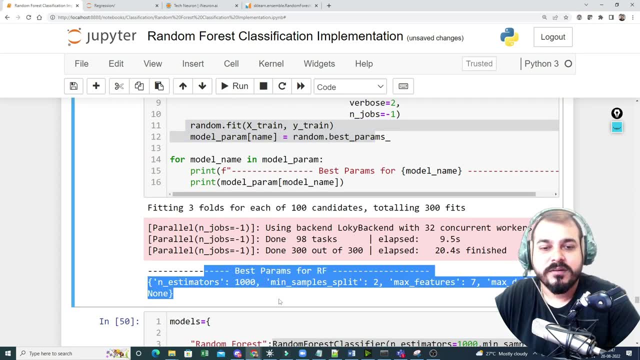 iteration and all we can play with it. and then we do the fact, uh, we do the fit on train by train and finally we got the parameters right. and once you execute this, we'll get the best param score right. and then i can probably use this and train my model and at the end of the day, see, 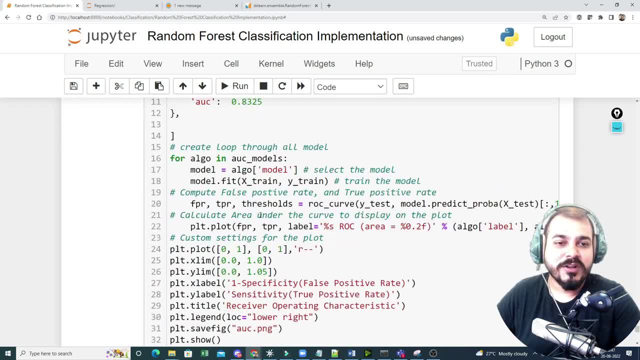 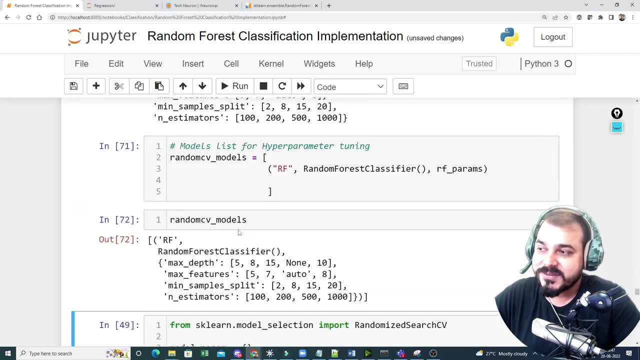 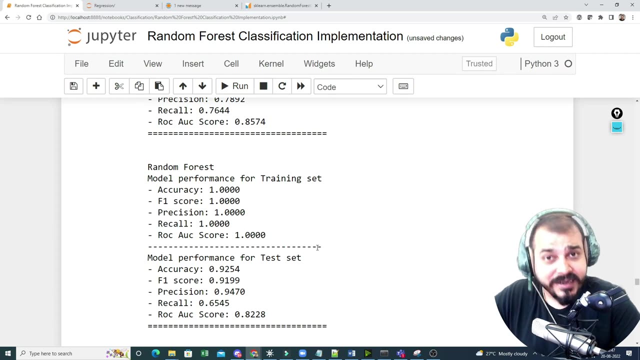 here also what i have done. i've made this roc roc score also automated, so here you can see how amazing it is basically coming. okay. so, and this all projects, right uh, this, this was basically developed from one of the fsds batch student, right uh, who are right now working in i neuron and since 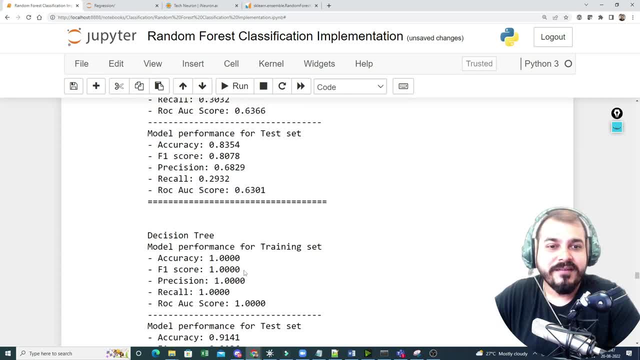 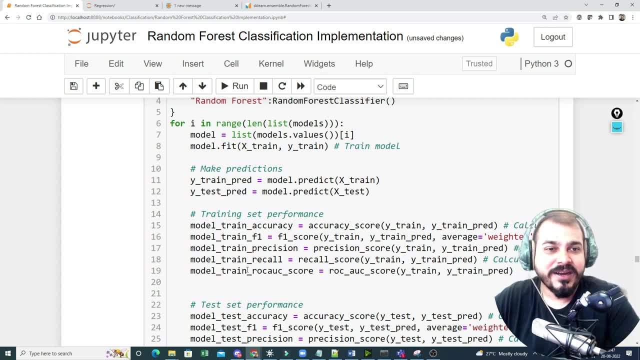 creating materials over here. you can see how beautifully they have actually explained it right over here. and if you really want this entire end-to-end project, just make sure that you hit like make it thousand. but this is how you have to do. tomorrow, if you want xg boost, i will probably go. 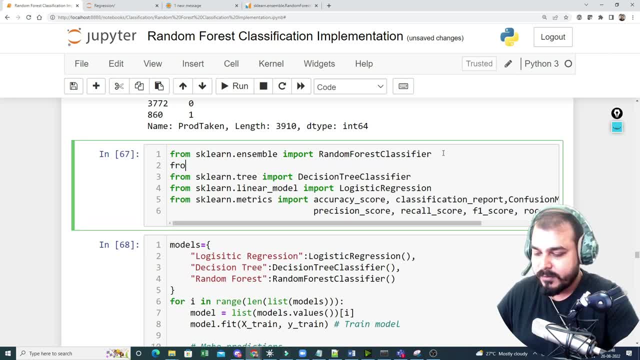 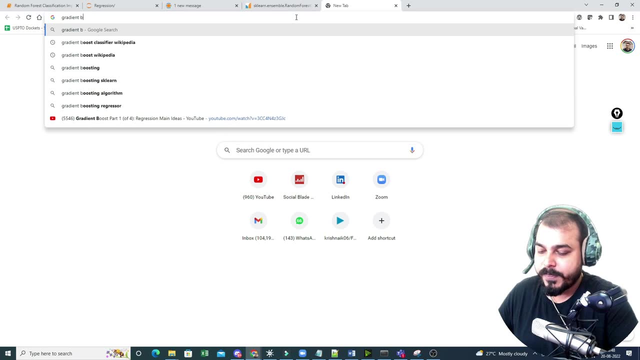 and search for xg boost. suppose i want uh gradient boost, so i'll write from sk: learn dot and symbol and symbol. import gradient boost classifier right, so i can actually go for a gradient boost. let's see gradient boost classifier where it is there: gradient boosting, ensemble gradient boosting. 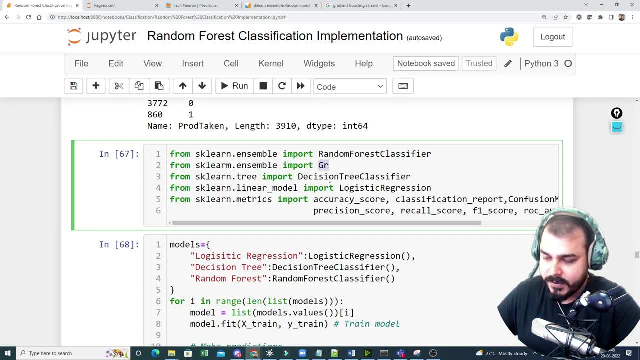 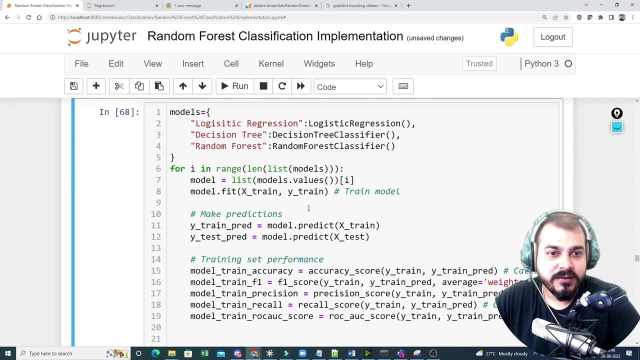 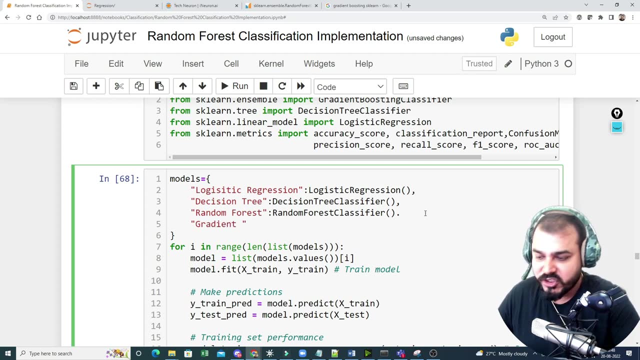 classifier. so i'm absolutely right. right, so if i probably go and search this now execute. so here you can see sk learn. now if i execute, just see this what is going to happen. all i have to do is that quickly just initialize this right gradient boost, that's it. i don't have to make any. 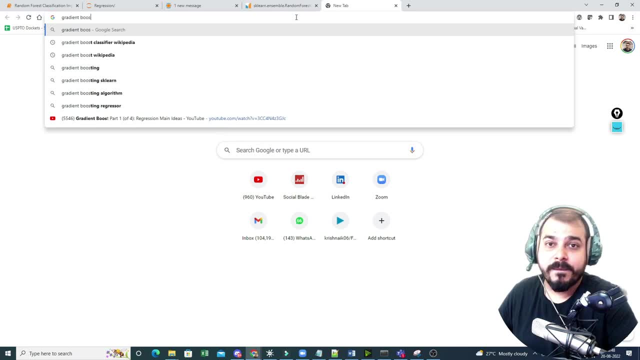 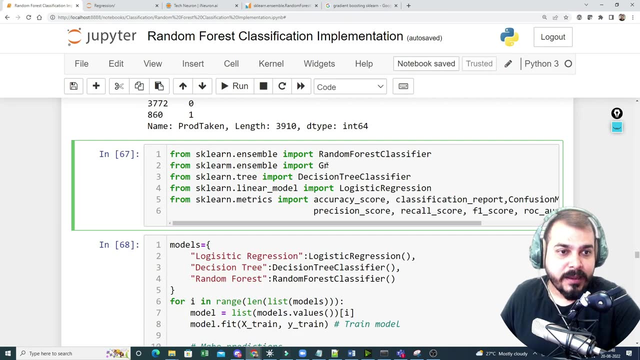 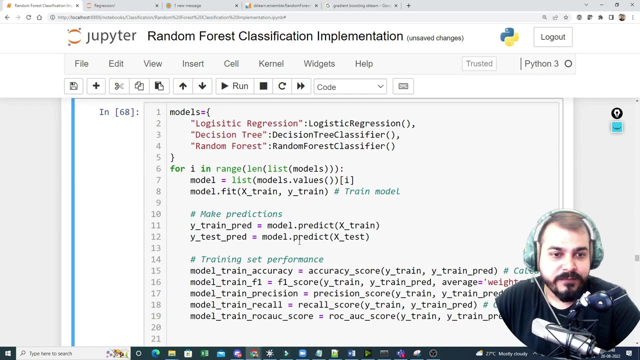 Let's see gradient boost classifier. where it is there: Gradient boosting nsymbol, gradient boosting classifier. So I'm absolutely right, right, So if I probably go and search this now execute. So here you can see sklearn. Now, if I execute, just see this. 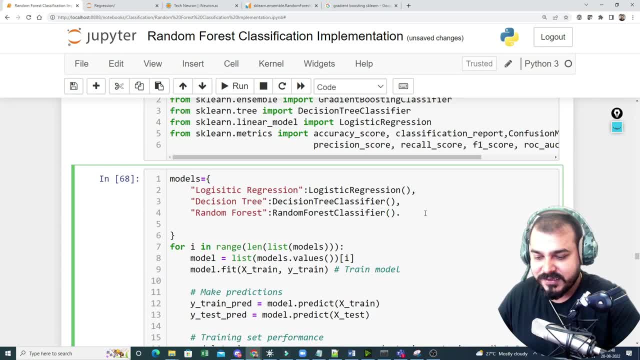 What is going to happen. All I have to do is that quickly just initialize this right Gradient boost. That's it. I don't have to make any change now With respect to training our model. And now just imagine if I probably create this as a function. 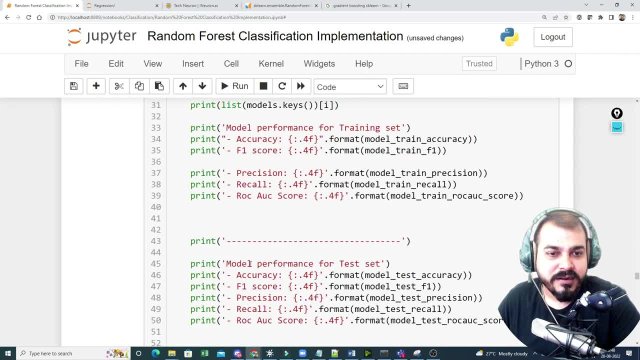 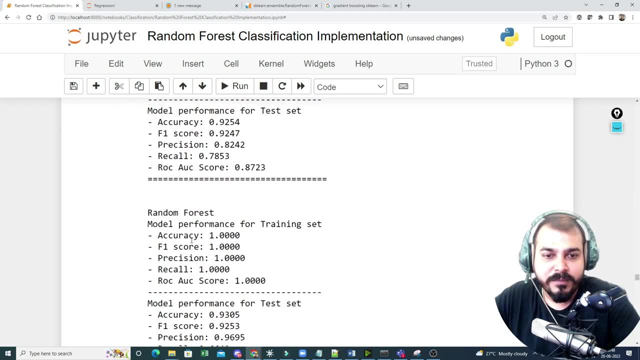 That's it. So here I'm getting some area Gradient boosting. Okay, I have to use some comma. I've used full stop over here. Now if I just execute it here, you can see automatically all the model trainings are getting. 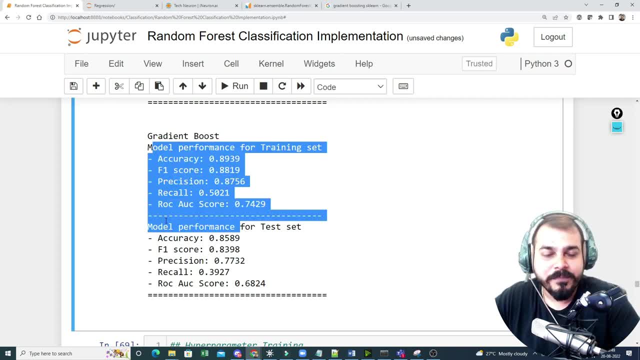 Now, here you can see, gradient boost is also not performing well. You are getting an idea right With respect to gradient boost. If you want to do AdaBoost, AdaBoost also you can basically do. Just go and import it over here. 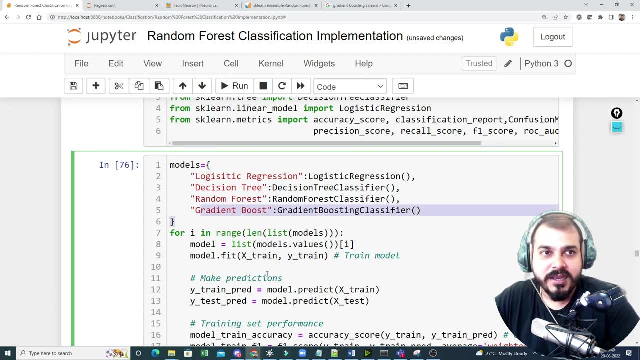 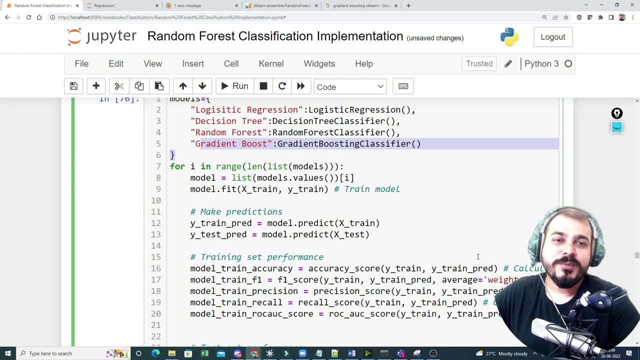 Just write the name over here and automatically the entire process will start. So I hope you got an idea that how you should basically train your model. Yes, this was the work of the students over here. I really want to make a quick announcement with respect to the Techneuron. 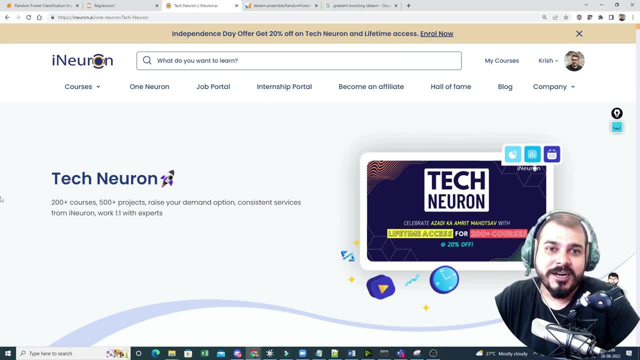 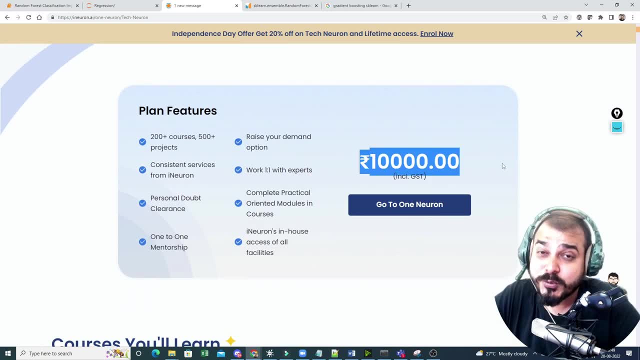 In iNeuron Techneuron. tomorrow is the last day to get the unlimited courses in Techneuron, along with all the live session for lifetime, at just the price of 10,000 rupees, And you can also use Krish20 as a coupon code to get additional 20% discount. 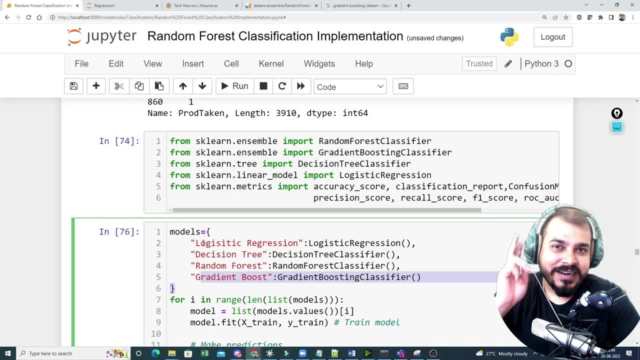 So yes, this was it from my side. Make it 1,000.. I'll try to upload this entire end-to-end video. Bye-bye, Take care And have a great day. 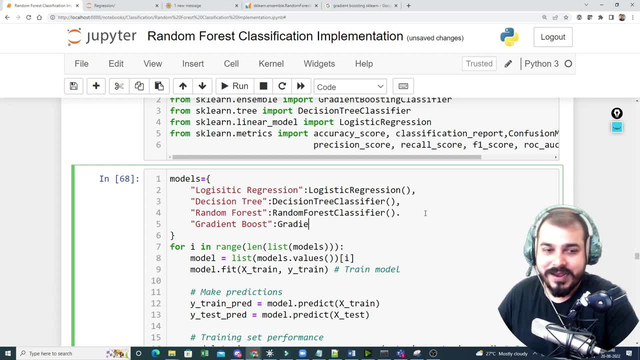 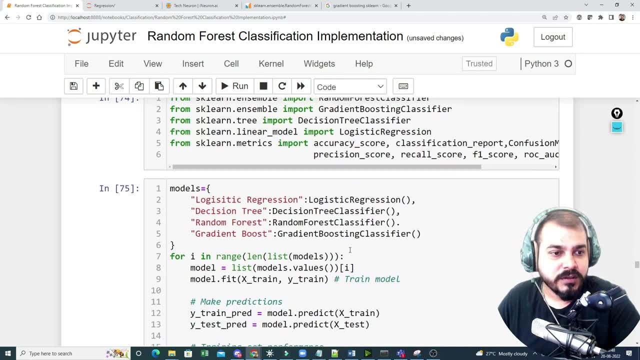 change now in with respect to training, our model. and now just imagine if i probably create this as a function. that's it. so here i'm getting some area gradient boosting. okay, i have to use some comma. i've used full stop over here. now, if i just execute it, you here, you can see. 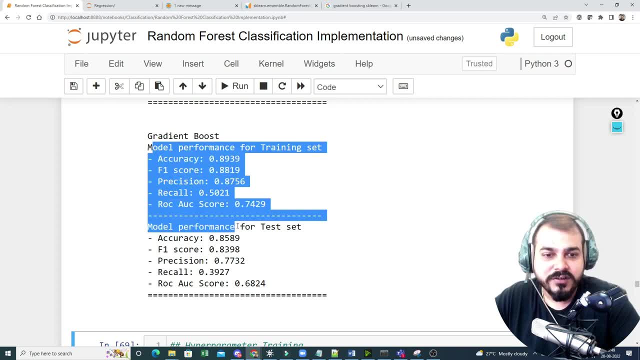 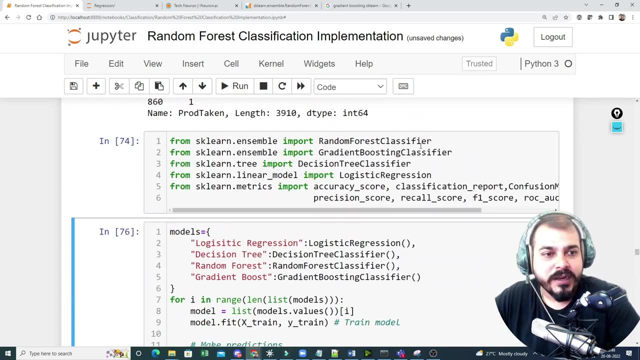 automatically. all the model trainings are getting now. here you can see gradient boost is also not performing well. you're getting an idea right with respect to gradient boost. if you want to do add a boost boost also, you can basically do. just go and import it over here, just write the name over here. 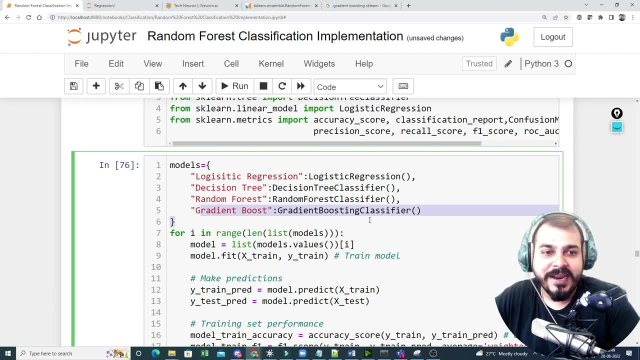 and automatically the entire process will start. so i hope you got an idea that how you should basically train your model. uh, so i hope you got an idea that how you should basically train your model. uh, yes, this was the work of the students over here. i really want to make a quick announcement.